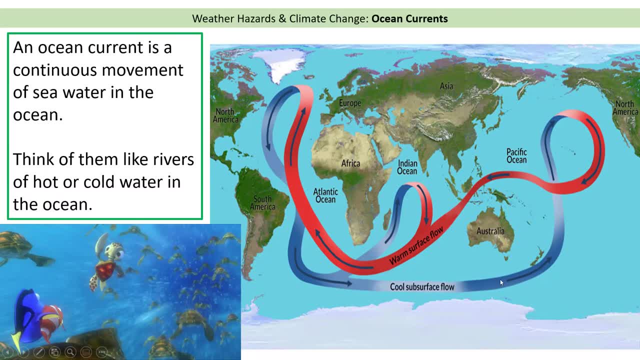 and that's this ocean current that I'm pointing out on the map over here. Okay, So ocean currents can be warm or cold, So the ones in red on here are obviously the warmer ocean currents and the ones in blue are the colder ocean currents. 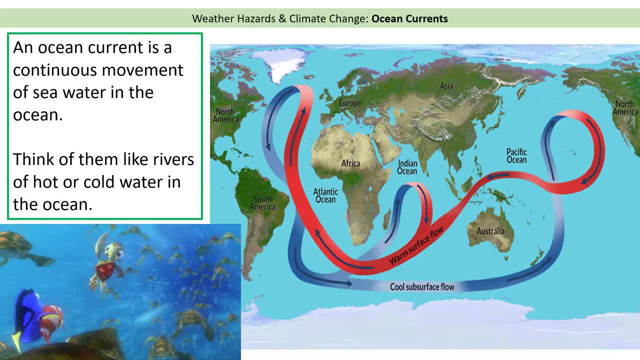 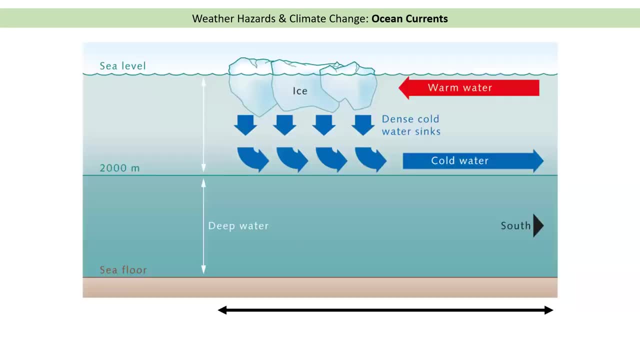 Okay So that essentially they're just conveyor belts or rivers of water and currents of water that flow around the oceans. Okay so how do they work? Why do we have these currents moving around in the ocean? Here we have a diagram showing. 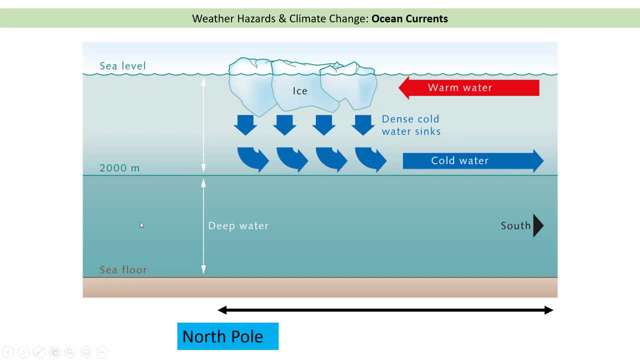 the ocean. On the left-hand side, over here, we've got the North Pole. So then this is the North Pole, over this side, on the left, and on the right-hand side, we've got the equator. Okay, we go to this in this direction. closer we get to the equator, okay. now the basic idea here is that. 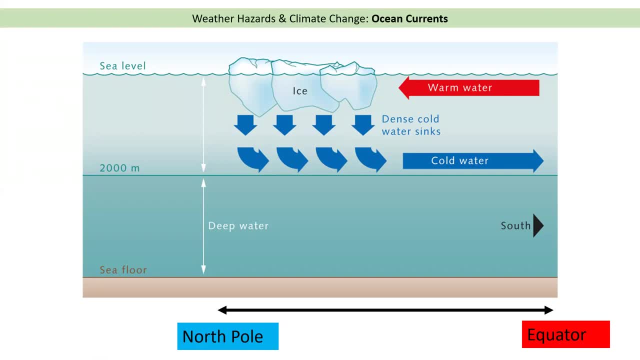 um, hot things rise and cold things sink, okay. and if you need proof of that, when you heat up water in a kettle, the water turns to steam and rises out of the kettle, okay. cold things, to the opposite, they sink, uh downwards, okay. so at the north pole the colder water is denser. it also has more uh. 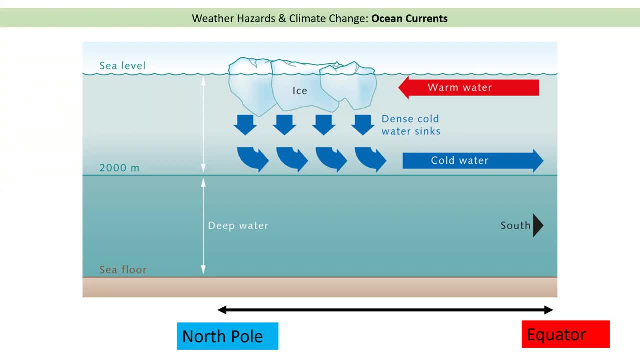 salt in it and that makes it denser as well. so the denser water, the colder water, sinks down to the bottom. as it sinks, it moves towards the equator, therefore it pushes the hot water out of the way, and the hot water rises and it comes back towards the north pole. okay, so we've got a bit of 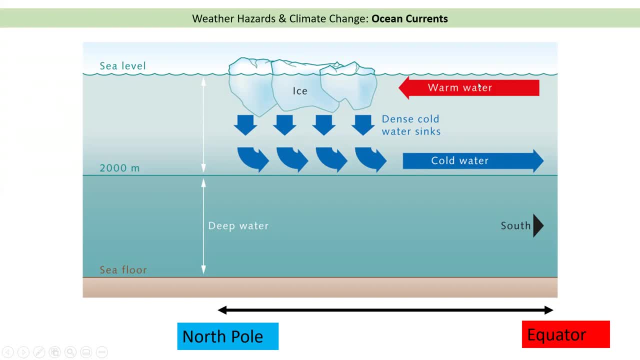 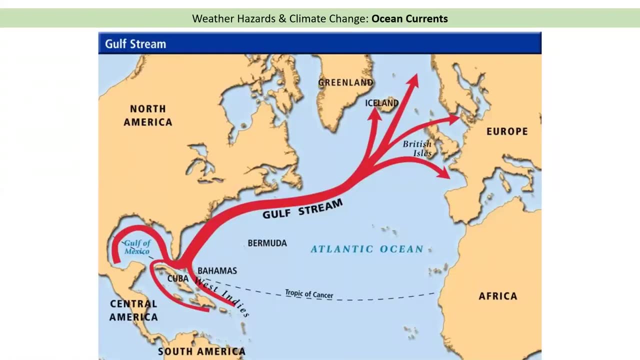 a conveyor belt here. cold water sinking, warm water rising, and that's the ocean current. okay, so the one we need to know about is called the gulf stream. okay, the gulf stream is the ocean current that affects- uh, the british oils and affects much of europe, in fact, and it originates, it begins, down here, in the caribbean- caribbean. 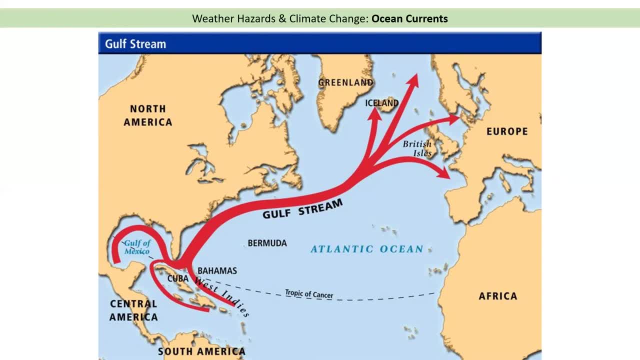 very warm water. um, if you want to go somewhere on holiday, uh, it's a great place to go. very, very warm seas around here and that warm water. there's an ocean current that comes from the caribbean and it flows up towards europe and it keeps europe much, much warmer.